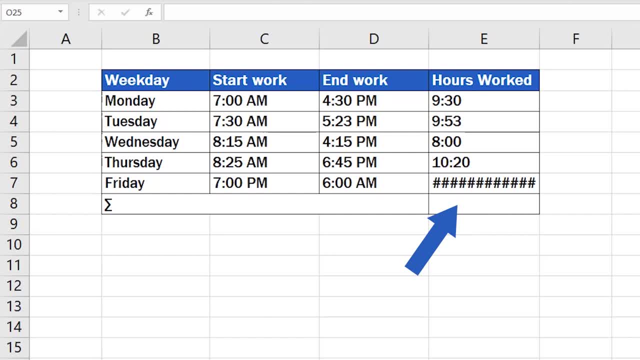 we need to use the same formula to calculate hours worked past midnight. Let's do this together. First, we need to remove the misfired attempt and, as usual, we type the equal sign in the cell that is supposed to show the result. 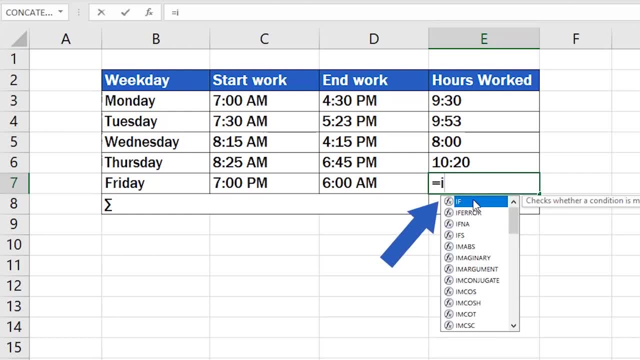 Now select the function IF by typing the first letter, I, and double-click on IF once you see the options. As you can see, for the function to work we need to enter the logical test first. Then we tell Excel what value to work with if the condition we want to work with is 1.. 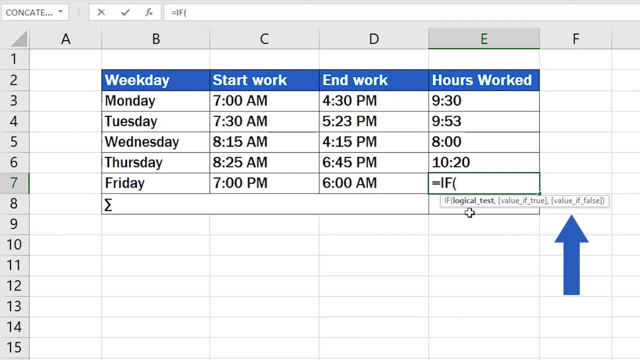 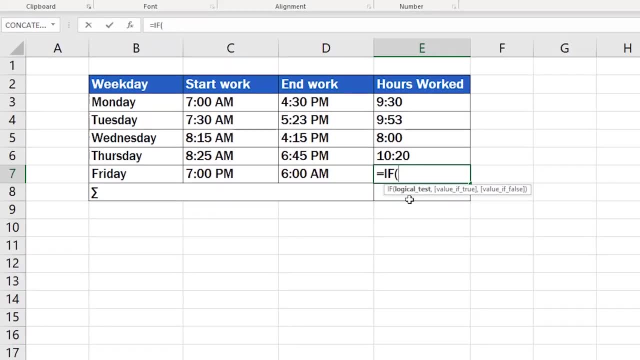 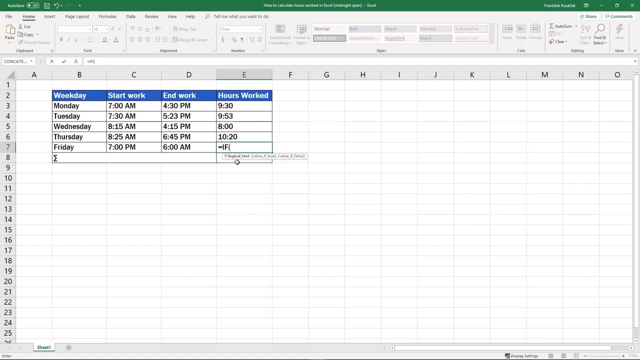 If the condition we entered is true and right after that we need the value Excel should take into account if the result of the logical test is false. In this tutorial, I'll guide you step by step through how to work with the IF function, in case you need to calculate time, More details. 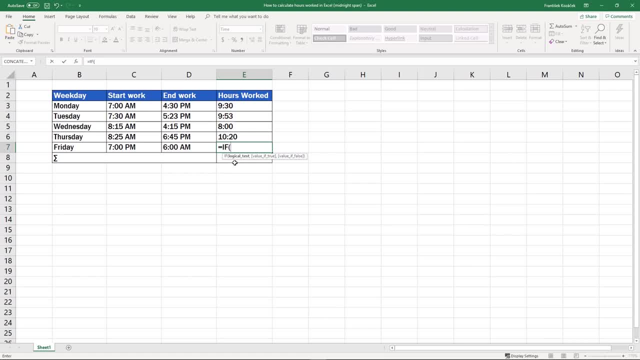 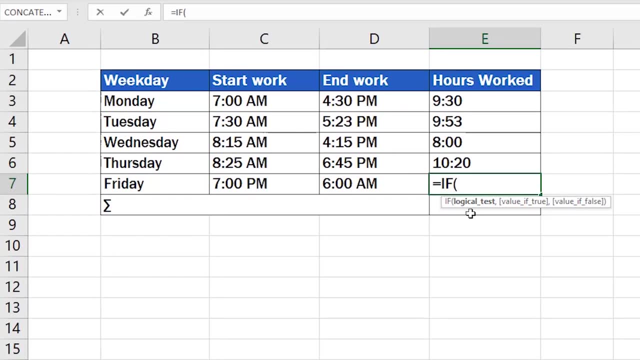 on how the function works can be found in the video on how to use the IF function in Excel. So, as for the beginning, we need to enter the logical test or condition based on which Excel decides what value to use in the calculation. After the IF word, we'll start typing out the 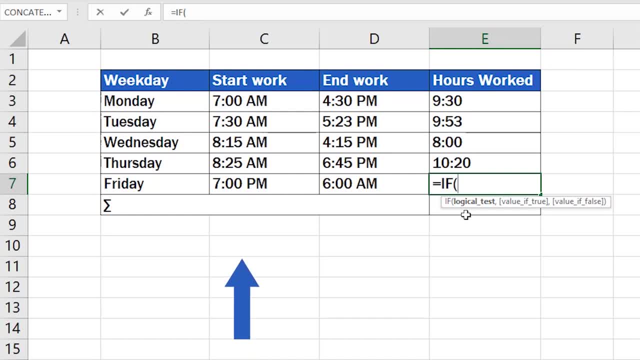 condition itself: The start work time- the value in cell C7, is greater than the end work time, the value in cell D7,, which is true for the working time that spans midnight. Type in the comma and we'll move on. Now we need to indicate that value. 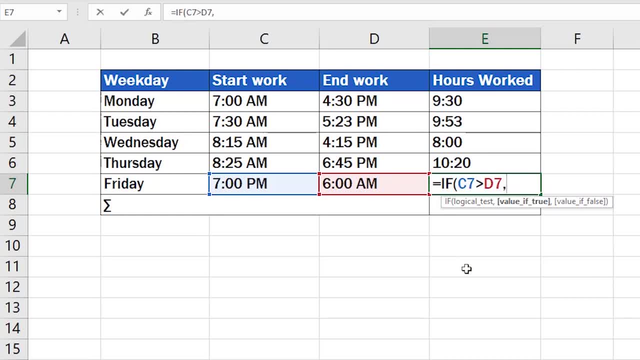 Excel should work with if the condition we entered is true. After that we also define the value for the situation in which the condition is false. So if the condition is true, we'll tell Excel that the work was finished the next day. We'll do so by clicking on the cell with the end work. 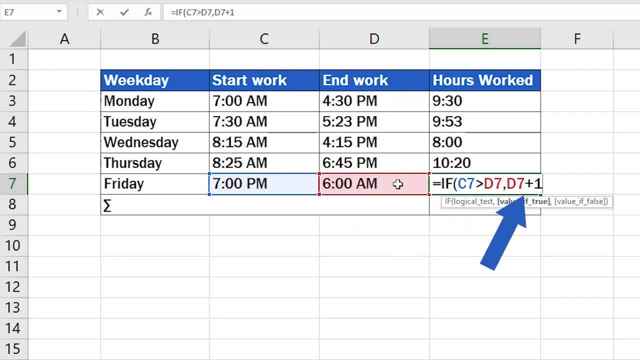 time data and we'll add plus one, which means that this time belongs to the next day. Enter a comma again. Now we can type in the value Excel will use if the condition we entered at the beginning is false. If it's false, we'll let Excel know that the end work time is in the same day. 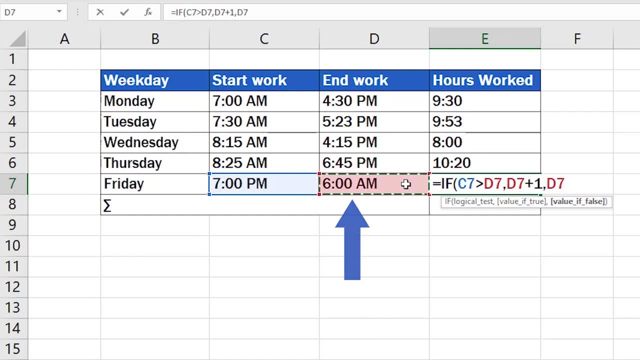 This is done by clicking on cell D7. Excel will then treat the time data from cell D7 as it appears as it was entered. This specific condition is false, for example, for the Thursday entry, because the end work time is not greater than the start work time. 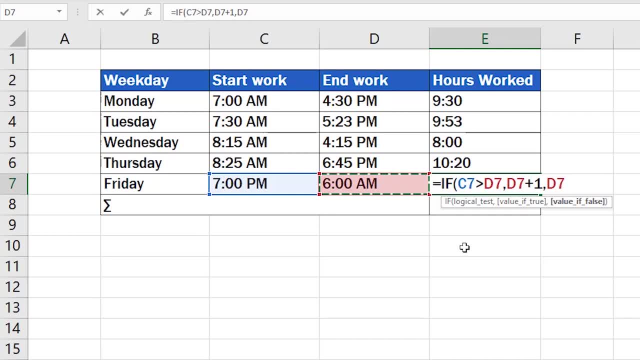 The formula we're now entering will be valid for all cases: hours worked on the same day as well as working time that spans midnight. We can do a quick test to check that together at the end of the tutorial. For now, we'll carry on creating the formula. 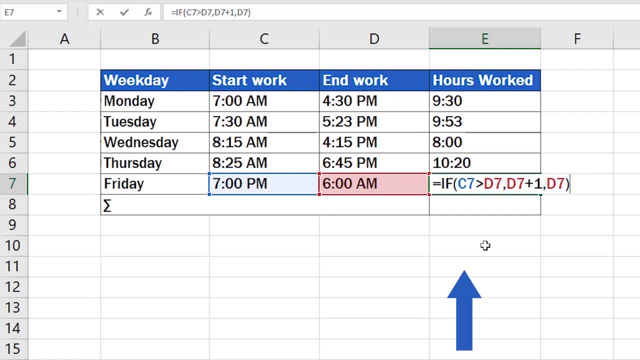 Close the brackets. Excel will now work as follows: If the value in C7 is greater than the value in D7, the value in D7 is from the next day. If this is not true, the value in D7 is from the same day. 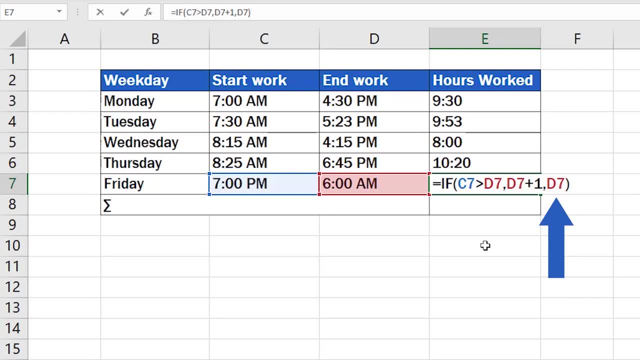 and Excel will use this value as it is Now. just subtract the start work time by using the minus sign, Click on cell C7 and press enter. That's it. You can see that now the calculated time- 11 hours- is accurate, And because you should be, 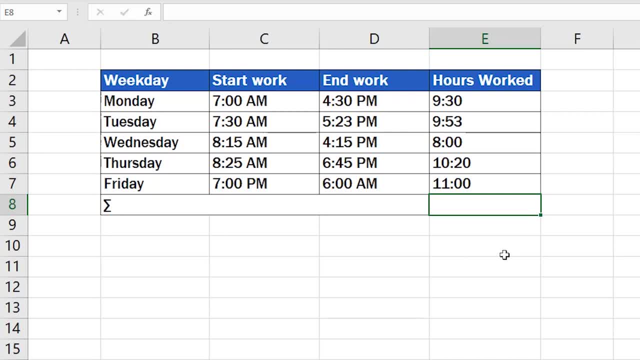 able to use the formula for the cases of hours worked past midnight, but also hours worked within the same day. here's to check whether it works. The formula in cell E7 can be copied through dragging the bottom right corner of the cell up through all weekdays, As you can see. 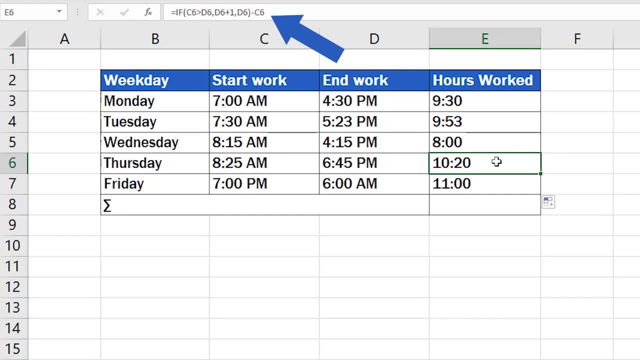 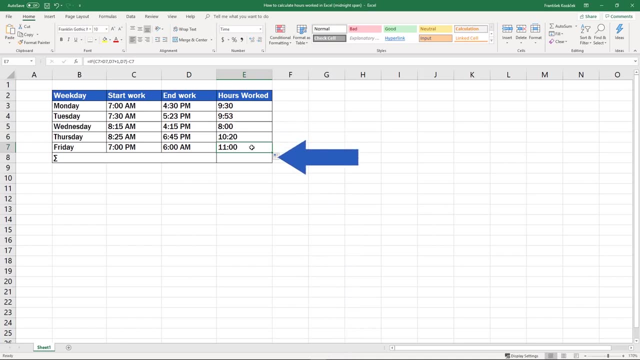 the formula is in all the cells and the times calculated previously didn't change. This means the formula works even in cases where the hours worked didn't span midnight. To see how we can easily add up hours worked throughout the whole week, watch the next EasyClickAcademy video tutorial If you're interested. detailed steps on how to. 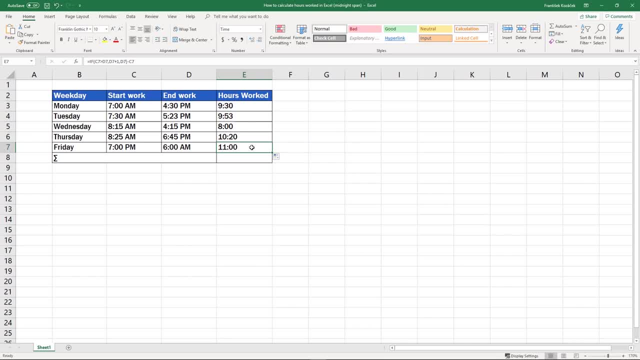 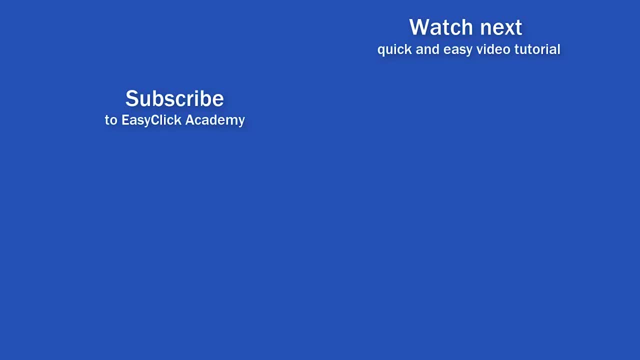 total hours, along with a solution to common issues when calculating time, are described in our video tutorial on How to Sum Time in Excel. If you've found this video helpful, like us and subscribe to receive more videos from EasyClick. Watch more videos that help you use Excel quick and easy.